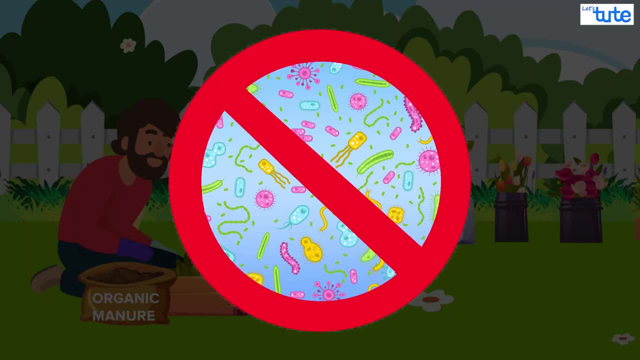 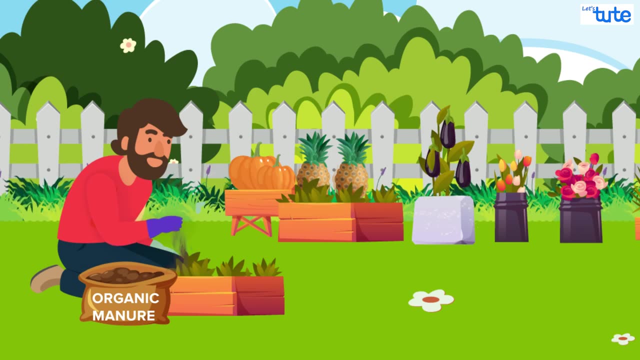 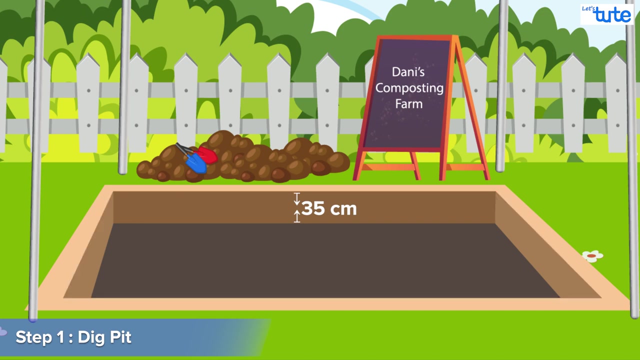 Danny does a similar process of composting, but instead of relying on microorganisms, he uses earthworms. Let's see how that is done. A pit of approximately 35 cm deep is dug in the ground in the shape of a rectangle. Alternatively, one can use a wooden box or a concrete pit of the same dimension. 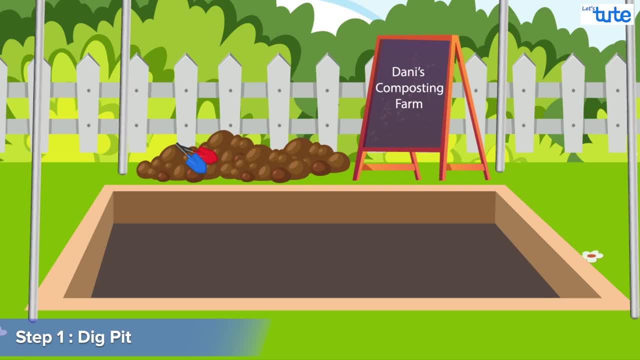 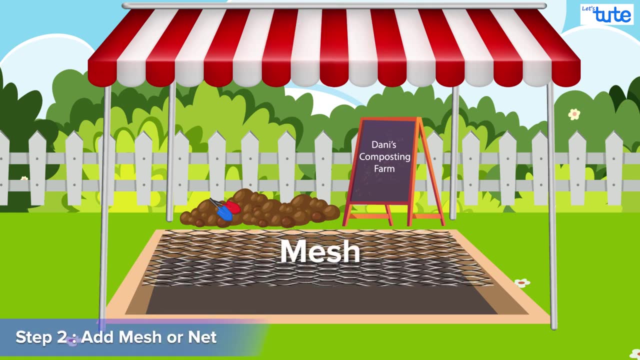 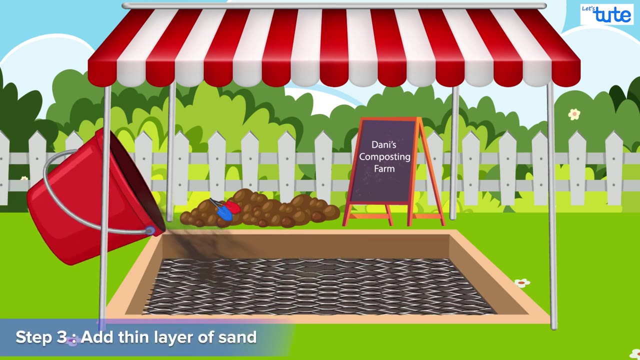 This pit should be dug in a place that is not directly exposed to too much sun. It should have a slight shade above A mesh-like thing, or a net is placed at the bottom of the pit. Alternatively, a thin layer of wood or a layer of sand- approximately 2 inches- can be placed at the bottom. 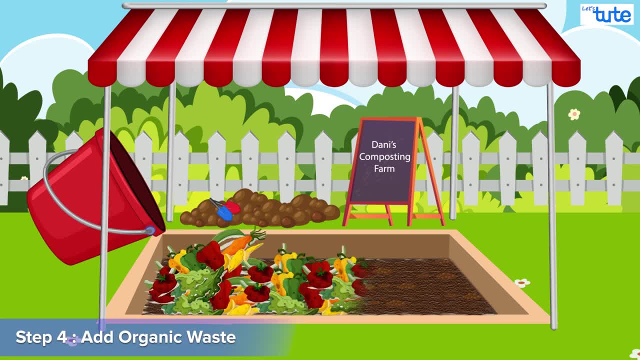 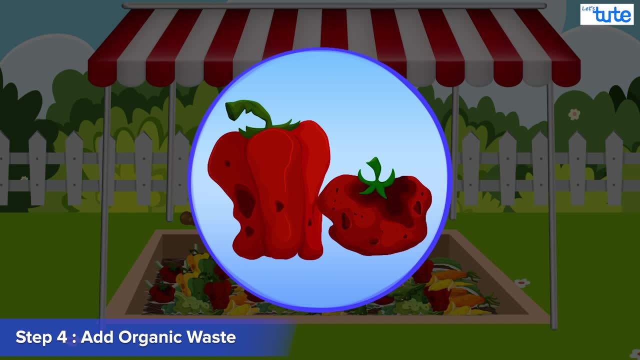 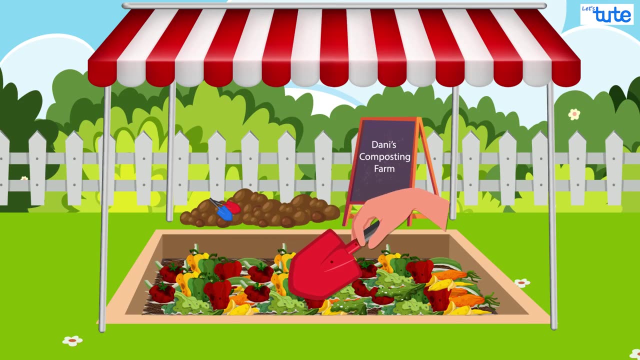 The next step is to add organic waste matter. By organic waste we mean all biodegradable wastes like vegetable peel, rotten fruits, other wastes from the kitchen, dried leaves, husks, cow dung, etc. Spread this across in a uniform layer. 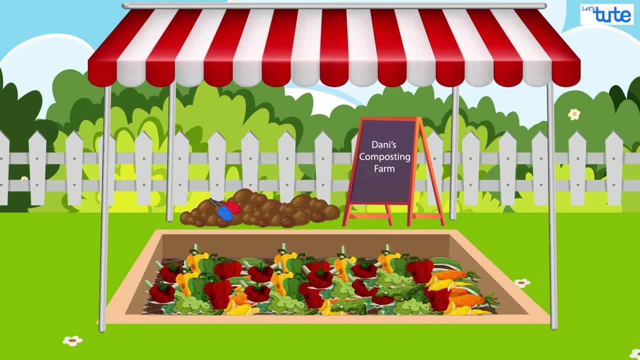 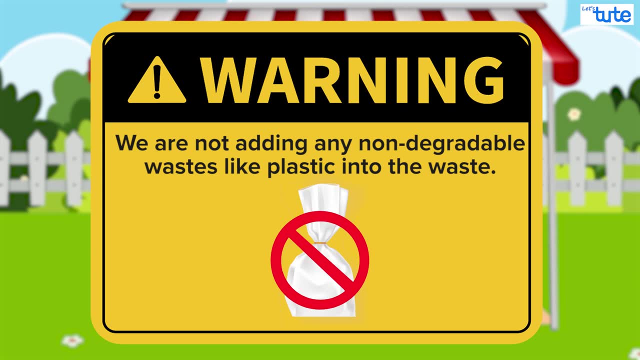 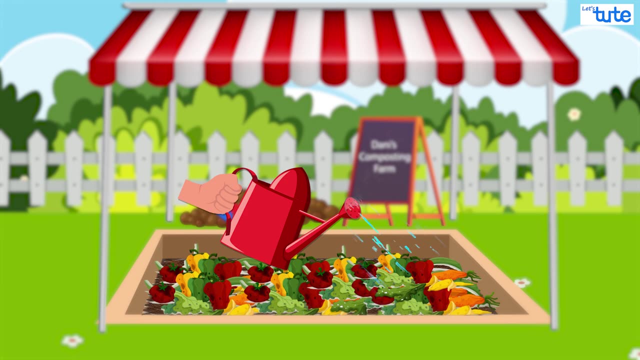 Do not press it, Make it compact, just spread it across. Also, make sure that we are not adding any non-degradable waste like plastic into it. It is important to keep the pit moist, so we sprinkle some water over the waste to just make it a little wet. 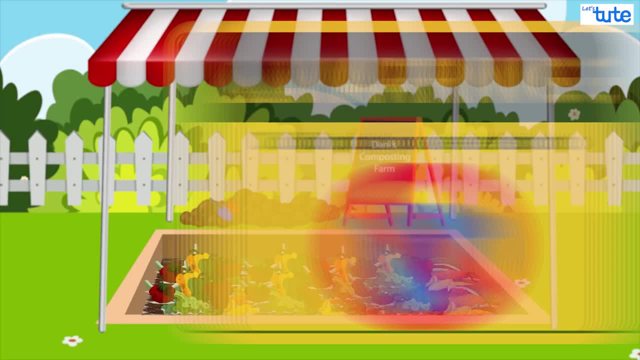 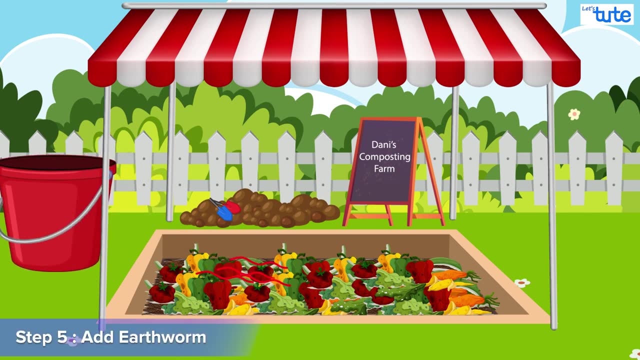 Please do not pour water onto this. Now is the crucial step, The step where earthworms are added to the soil. A special species of red earthworms, Isina photida, is used. You might be wondering why earthworms? 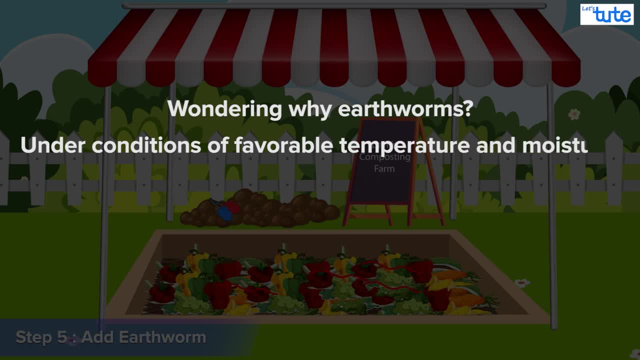 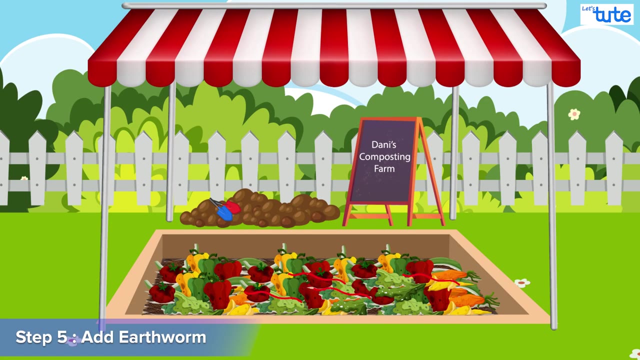 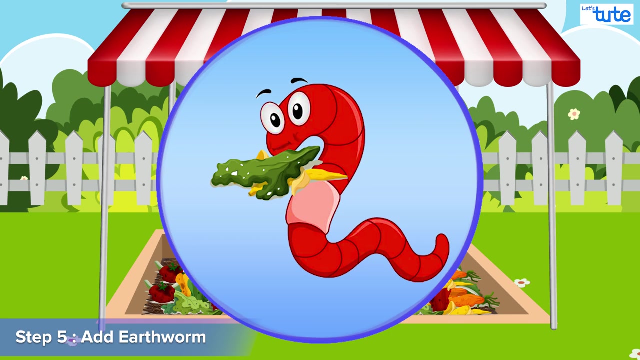 Well, under conditions of favourable temperature and moisture, the earthworms consume this waste matter and convert them into simple form, or say, decomposes this matter to form compost. These species of earthworms are non-burrowing, meaning they stay in the layer of the soil and break down this waste efficiently. 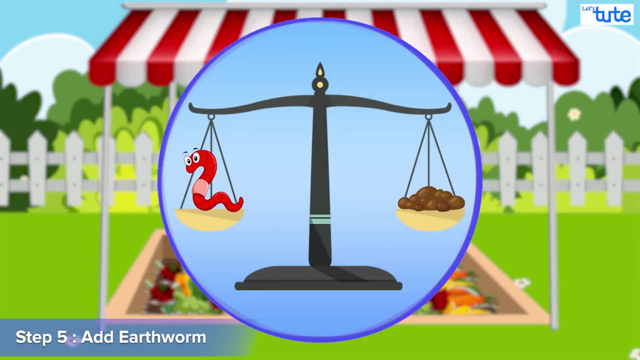 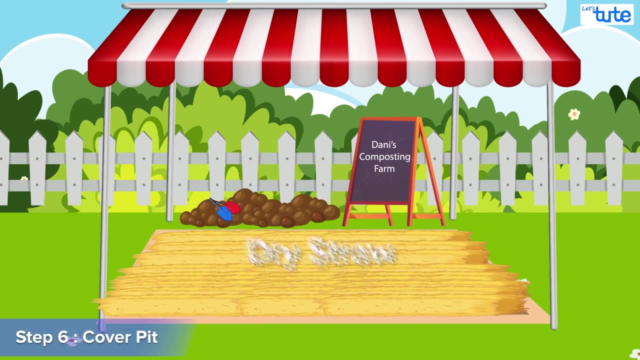 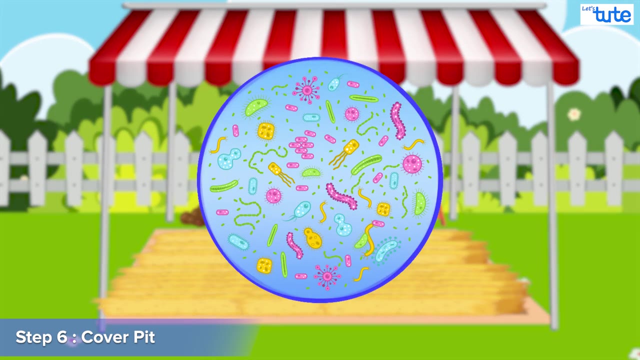 They are capable to produce waste equivalent to their body weight. Amazing, isn't it? Once the worms are laid, the pit is then covered with dry straw or gunny bag. Covering the pit is very essential, as during decomposition it could be a site for disease-causing organisms and germs.